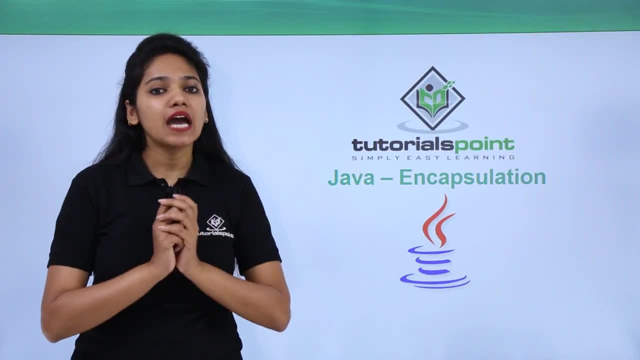 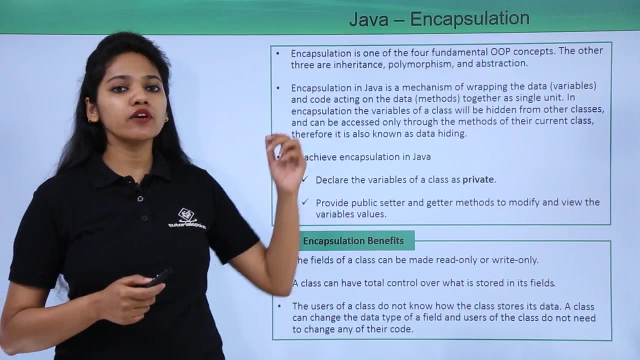 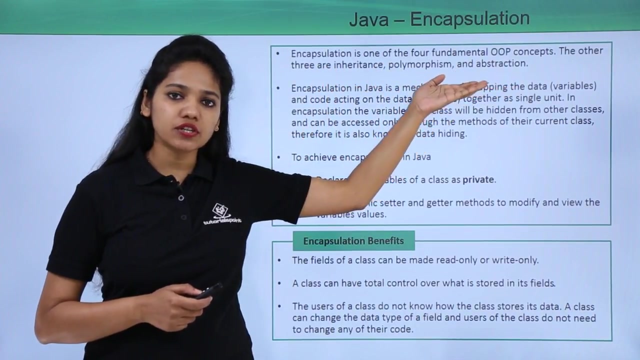 which is much more related about how you program and how do you make your data, members or variables available for others. It is one of the concepts in OPE. The other three already we have seen, like you have inheritance, polymorphism and abstraction. But what is encapsulation all about? 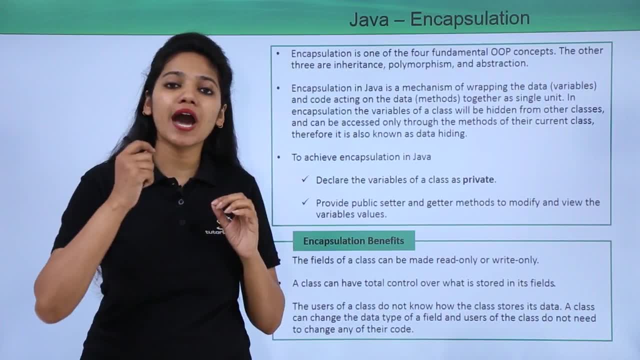 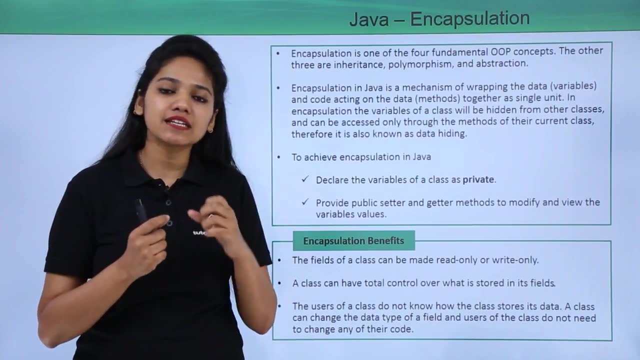 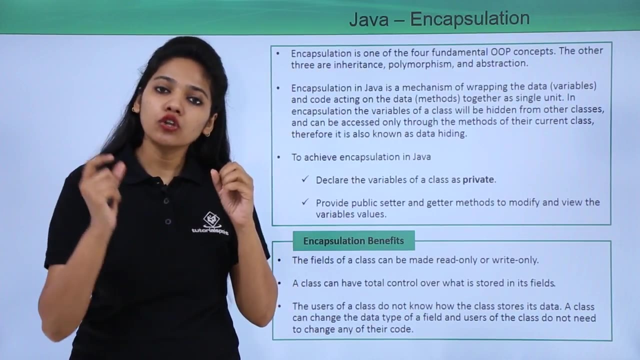 And encapsulation is nothing but which allows you to hide the implementation details of your class. What do you mean by that? So now you have certain data, certain methods of your class, So it allows you to wrap the data and the method or the code that acts on this data together. That is, you wrap the data. 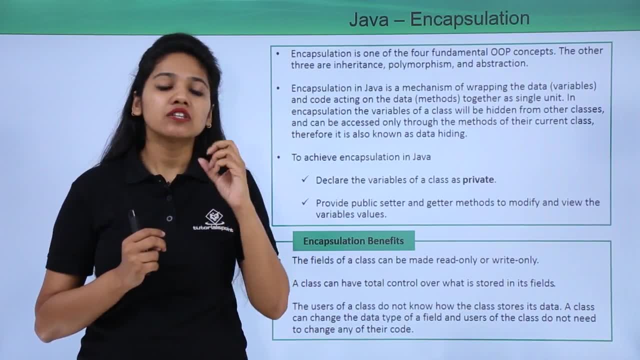 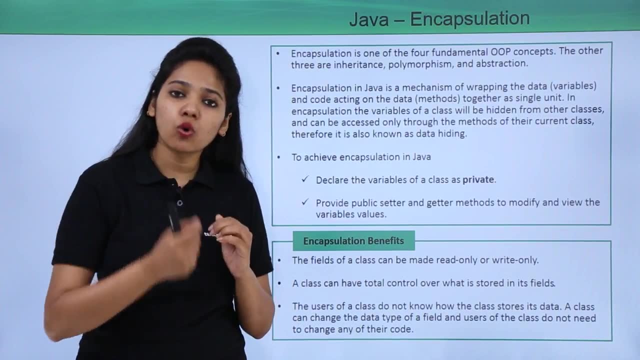 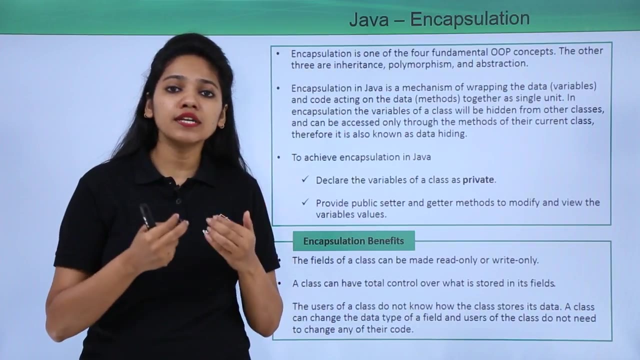 and the data method in a single class. Now, what happens to this single class To whom all is visible? A user? can a user see the coding, the implementation? No, The concept of encapsulation. say that please tell the user what does this class do, but do not provide the details to. 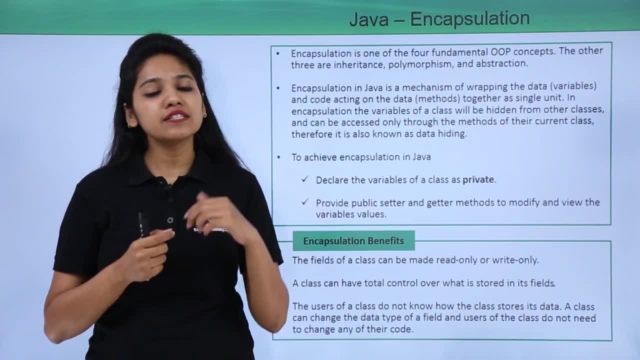 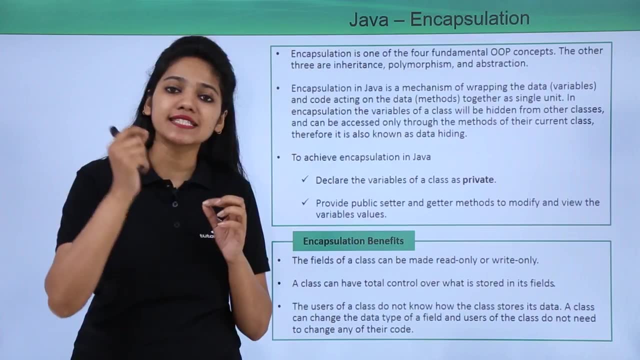 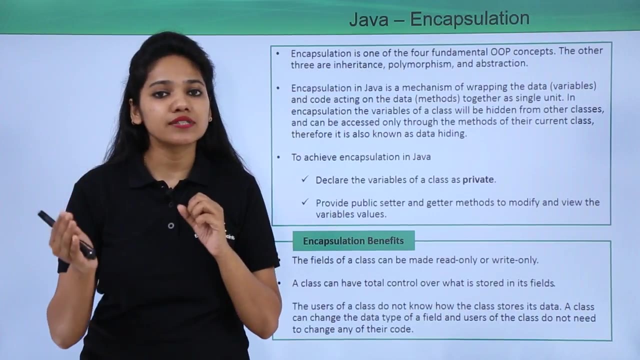 the user. How does this class perform? That is, which is a very general example of a capsule: when you have- you do not know what are the ingredients or the molecules inside- that just have. It means it wraps the data, which is that you secure your data from the outside world. What it says here: 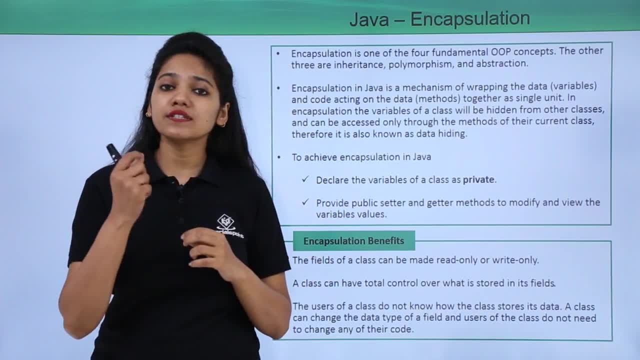 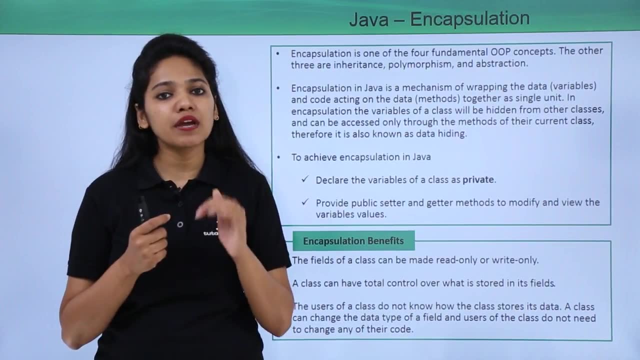 is that to achieve these kind of a concept? what is this concept? Now, you have declared certain variables and methods private. By making these methods or variables private, you are able to make these methods private. It will not be visible to the outside world. But what in? 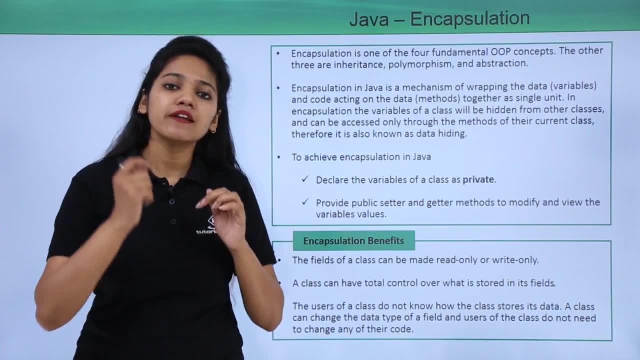 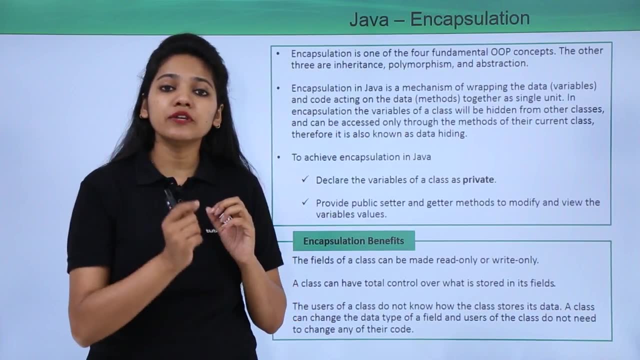 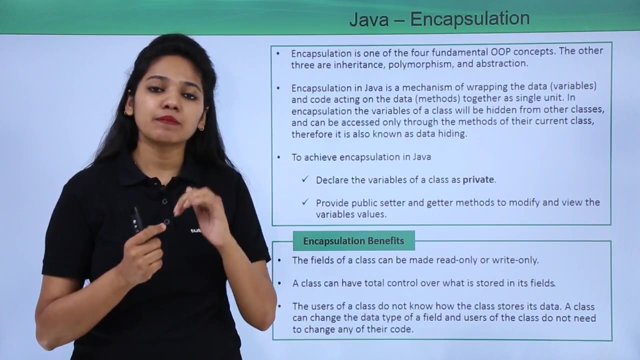 certain cases where you want these methods and variables to be accessed, that is, you want to access these private method and variable. In those cases you need to set public getter and set of methods for these private variables to be accessible to the outside world Again. 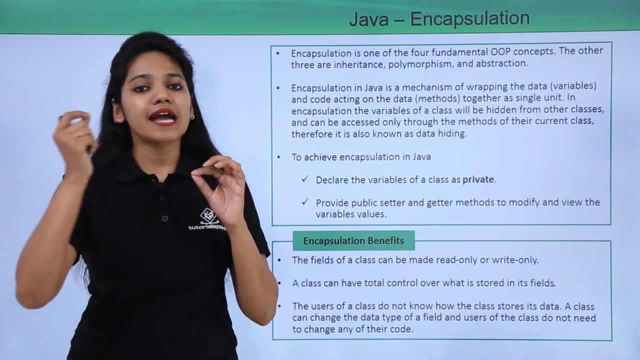 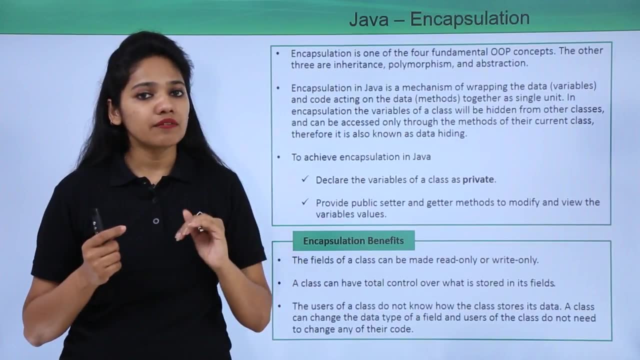 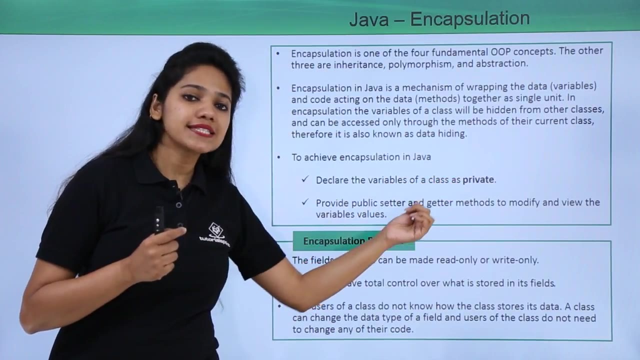 repeating: if you want these private variables to be accessed from some other class, then you need to set public getter and setter methods for each of these private variables. That is what it says. You need to declare the variables as private and then set public setter and getter. 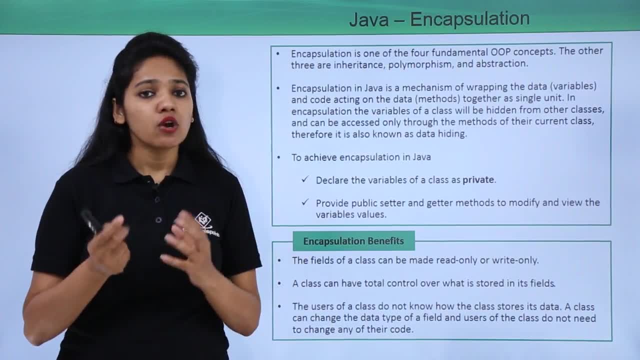 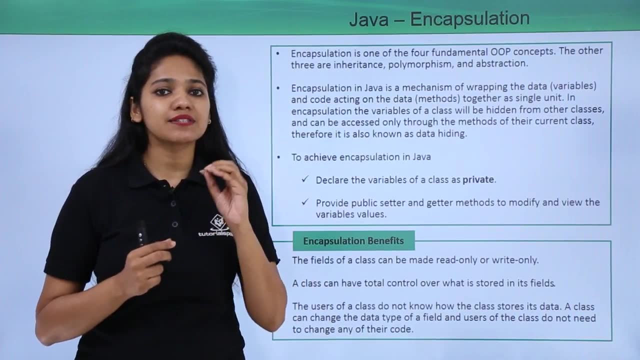 methods for these variables to be accessed outside? What happens with this? What kind of a control can you have over these classes? If you want, you can make them as read, only by just making as private, and when you want to make it as write, only you can provide certain public. 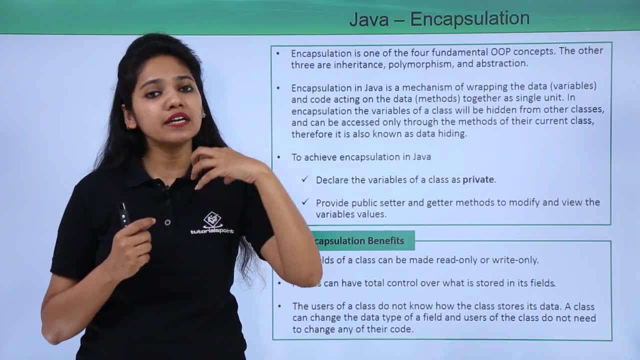 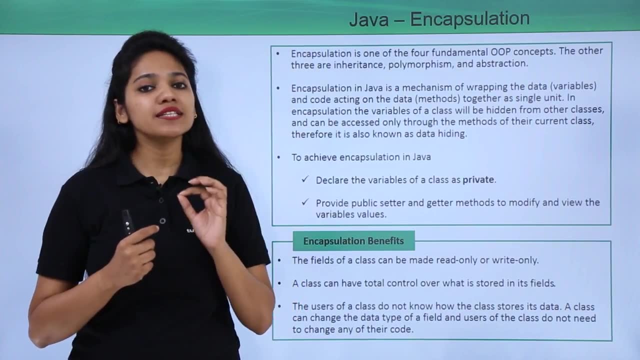 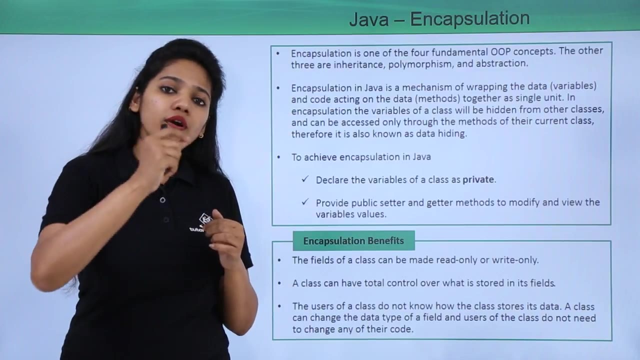 getter and setter method, and you can have a better control by using these kind of a methods. How Now for new example? you have created a class where you have certain integer, that variable or value, What you want. The outside user should know what that this class do, but should? 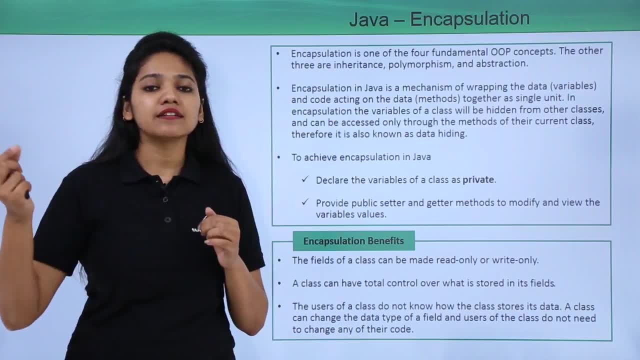 not know how this performance has happened. That is, according to the user, the value that the user is trying to enter is an integer value, But at the back end, what they need is a set of natürlich Super irrelevant. So let's try this. If we go into includes: 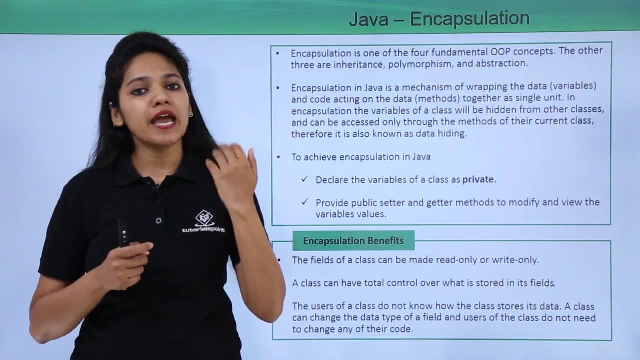 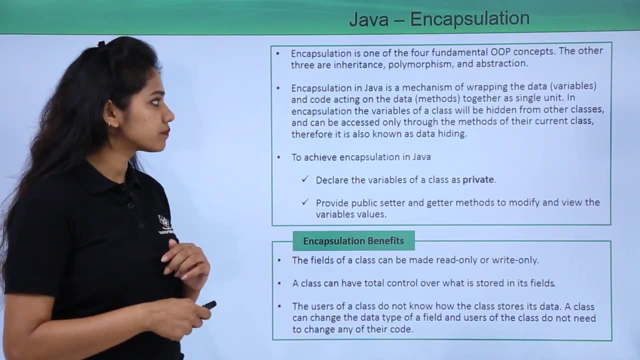 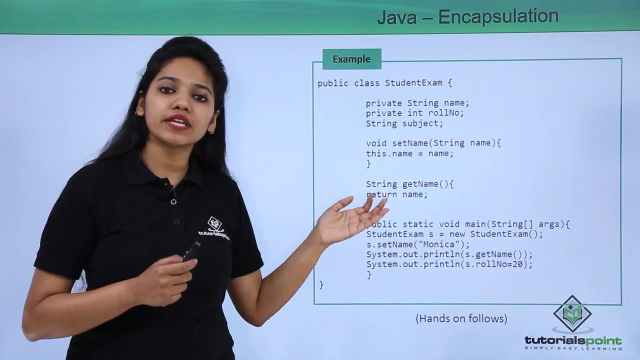 backend you can change the integer value to long, double and so on. So it means when you change the field value that will not be known to the outside user. So this is one of the examples where we have created a class called student exam and declared certain variables. 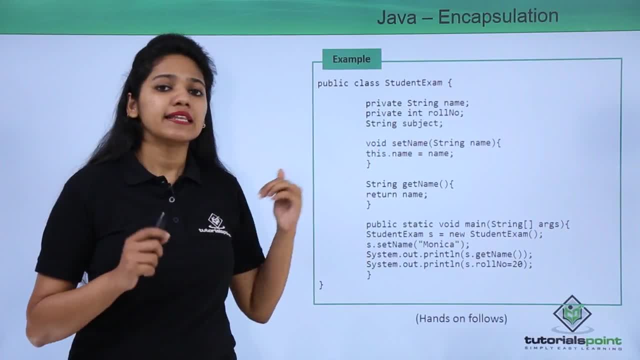 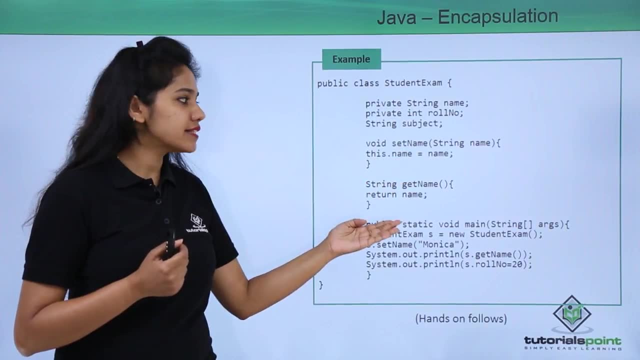 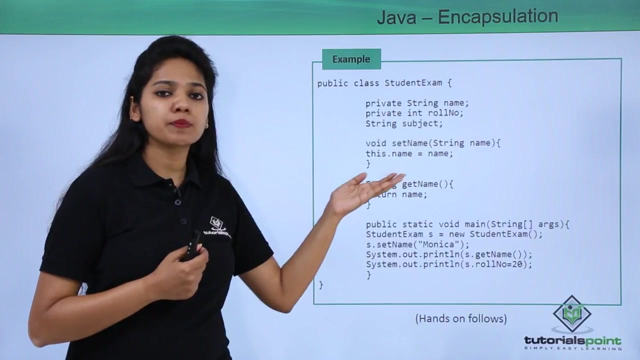 which are certain are private and the rest one are public. Now, in order to call these private variables outside the other class, you have set certain public getter and setter method. If I have not provided any access modifier, by default it is public. Therefore, I have specified certain getter and setter method for one of the variable and in the 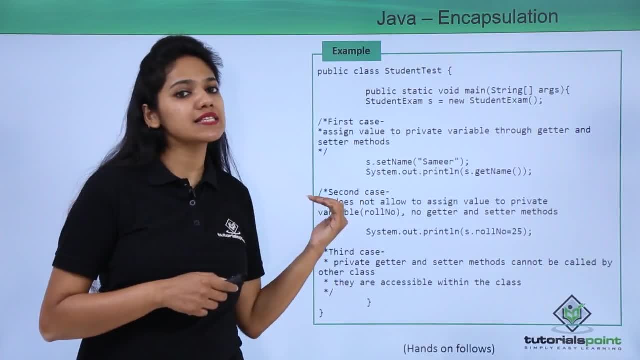 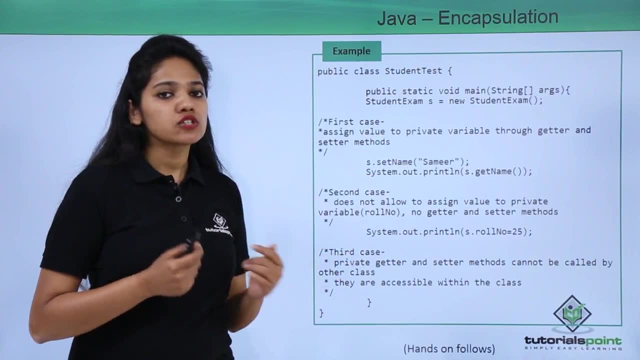 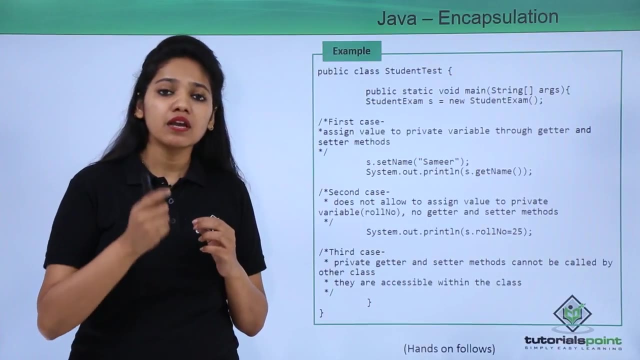 next, this case in this class, where you are trying to access the private members or private variables or public variables. what are the certain course of action happen. So let us execute this program in practical to understand what happens when you are trying to call a public variable, a private variable. 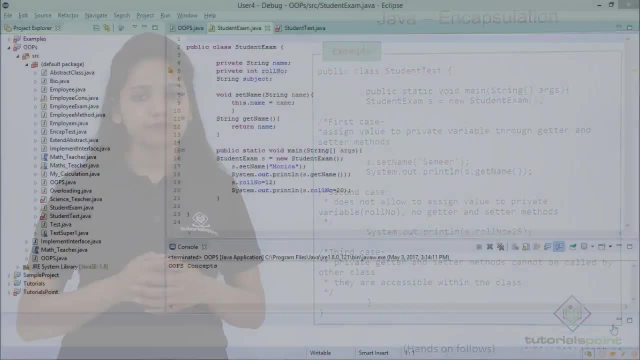 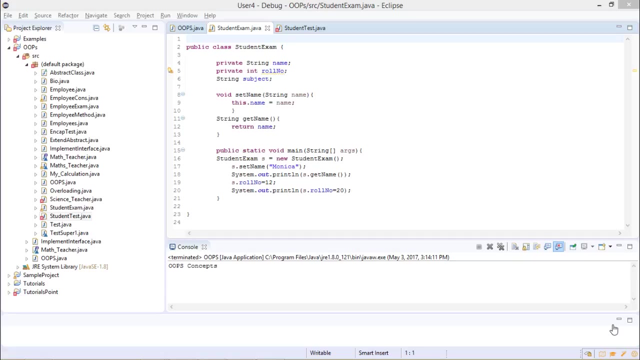 By now we know what an encapsulation is all about. Till now, whatever the programs that we have written, we were trying to bind the data and behavior in a class. That is what all encapsulation is all about. But let us see with the help of an example, if you would. 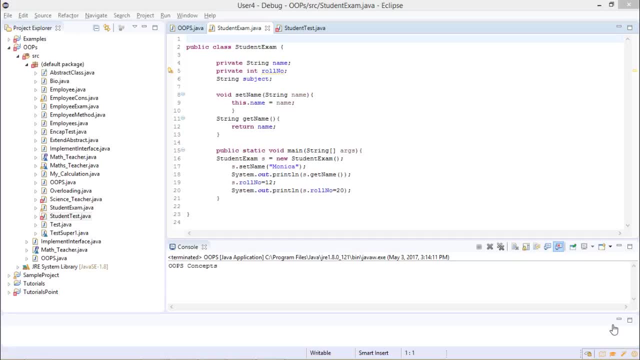 want to bind the data and then call into another class where the variable or the methods are of private type. So will you be able to not, or will you be able to bind this kind of a data and the behavior together or not? So we have created a class called student exam, in that we have created 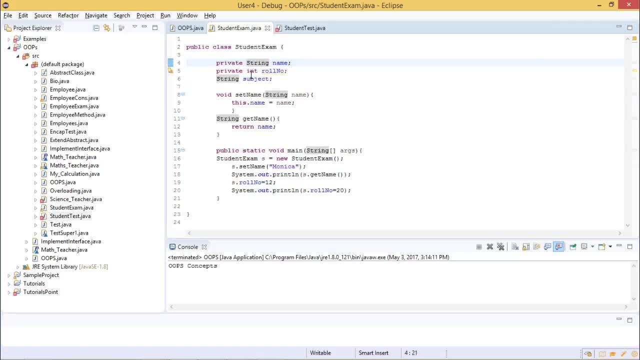 three variables, two of string type and one for integer type, where string name and string subject, where string name and enrolled number are of private. and these private variables, normally a private access modifier rule says that the variables or the methods that are third declare private will be accessible within the class. but in the concept of inheritance we 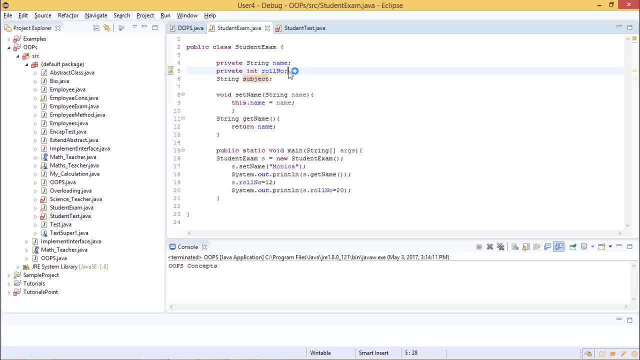 need to see how can you can access the variables of the methods which are declared private. so in this class we have created a method called set name and get name, where set name is nothing. but you're trying to get the value of the name from the main method and store it in the string. 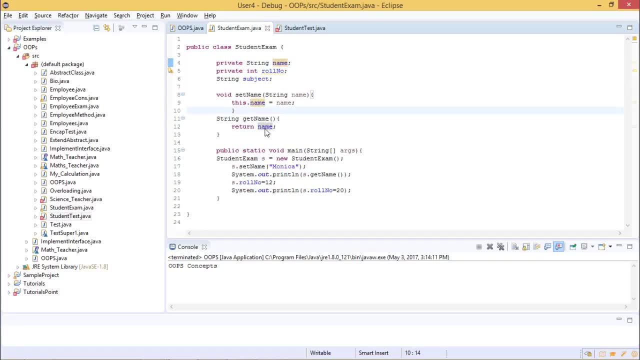 variable and that again you can return this value with the help of written keyword through get name method. so in the main method, first we have created an object reference for this class and this object reference will help us to call the set name method. in this set name we need to: 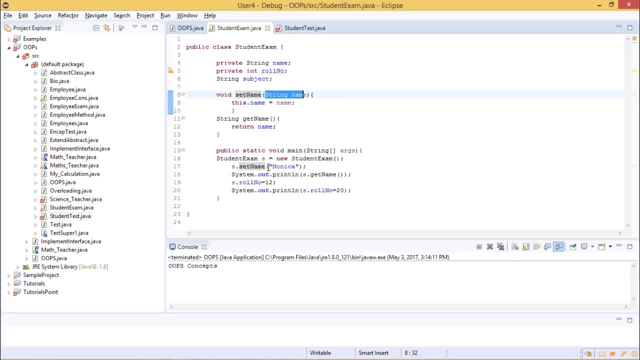 provide a variable value that is string type. so we provide the name as monica and then when we are trying to display- we need to get this method- we are trying to display the name of the variable in this set name. so this is how you think we can access the private variable in your class. 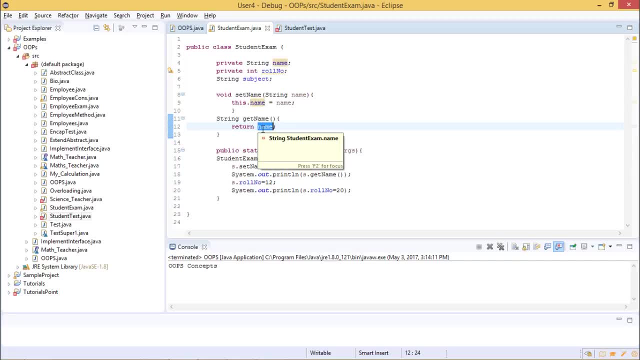 so in this class a got var and the under screenshot is aboutgerly. we are trying to come to the set name method. we are trying to get the value from get name because you are trying to set the value, that is, you call the value and then you store the value and then you have to return the. 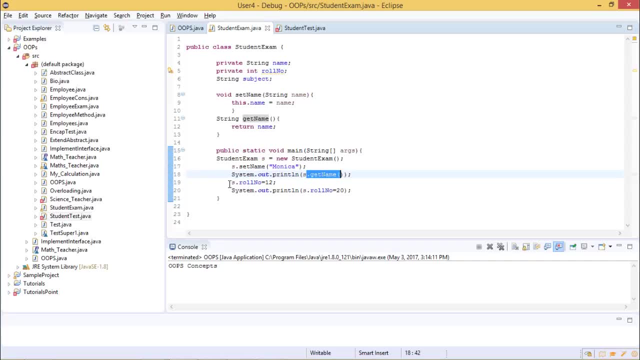 value and the return value is from name and that is coming from getting method. so you write the object reference, that is s dot get name right. so this is how you can access the private variables, finally printing that value. So let us execute this program. As you can see this program first. 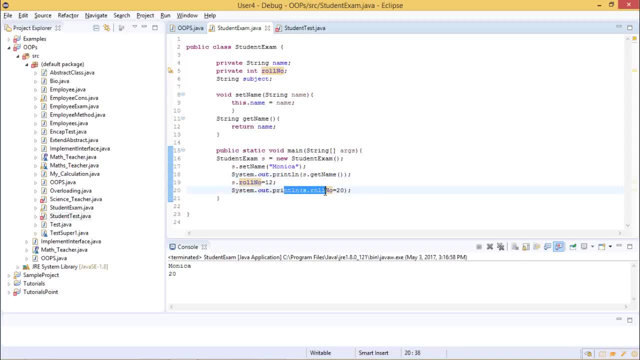 prints the name as Monica and then the roll number as 20 at not 12.. If you would have provided here system dot out dot println, that is, under the system method, then the roll number would have been 12, but we are trying to print only roll number as 20.. So let us now see how can you call? 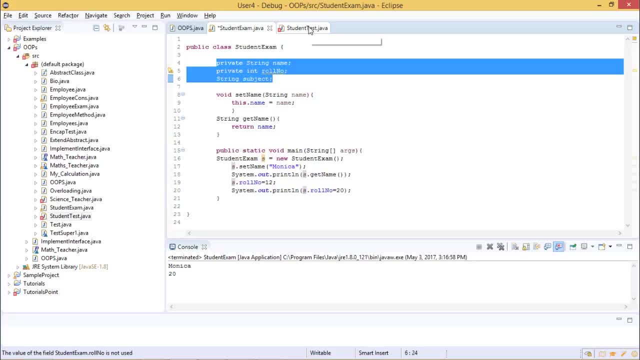 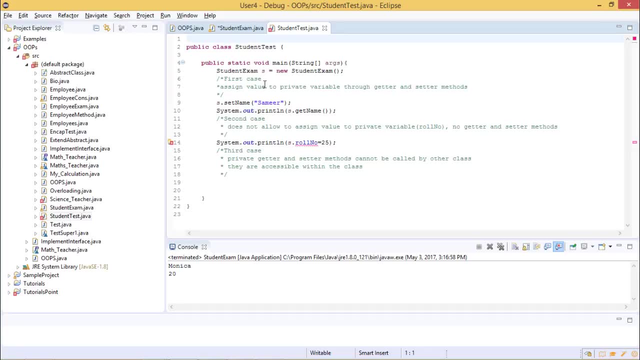 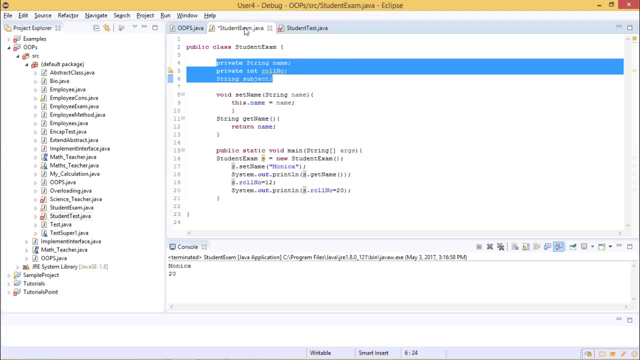 these private variables into another class, So we have a class called student test. okay, and if you want to call them here, what are the possibilities that we need to understand? So, in the main method, I have created one object reference for your student exam class, right? So we just say that. 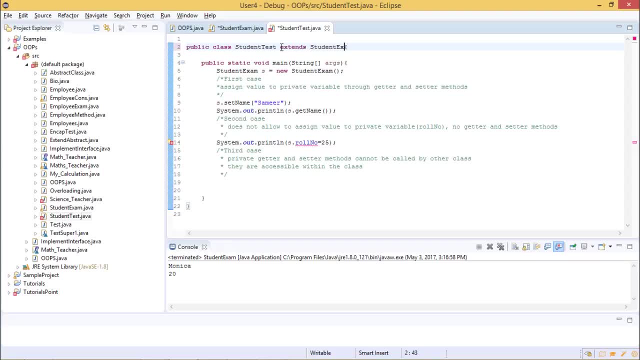 we want to extend the student exam- or you can directly create the object reference for this class. The first case would be that, if that is, assign value to private variables through getter and setter methods, That is, if you want to override the value or if you are trying to call the value, how can you do that? If the variable 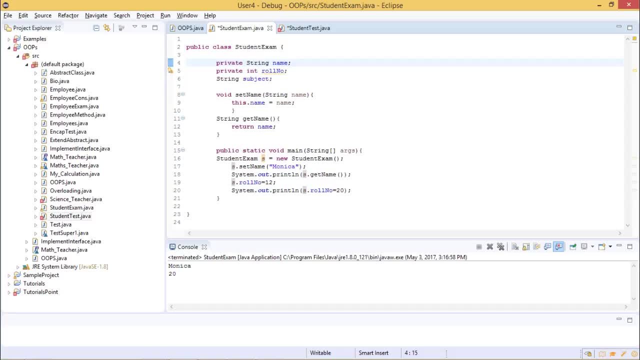 are private. if any variables are declared private and you want to access these variables into another class, then these variables should have public getter and setter methods. If you have not specified any access modifier, it means they are public getter, So it will allow you to call the private string name variable because it has its getter and setter. 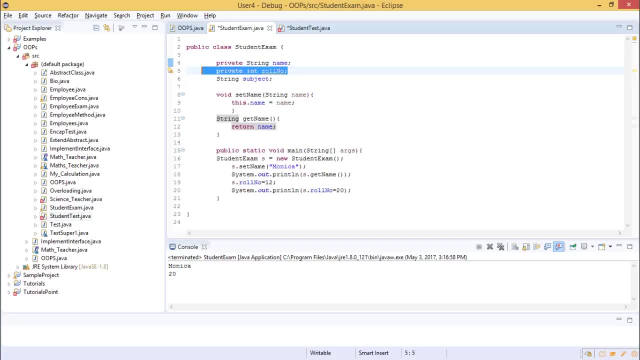 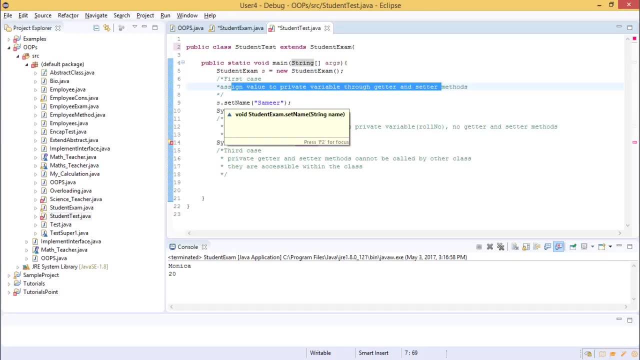 variables, the methods. but int roll number will not be able to call because it is private and it does not have any getter and setter methods. So we write sset name. we can set the name as semi now and we can print the value. This is how you are overriding the value. In the second case it does. 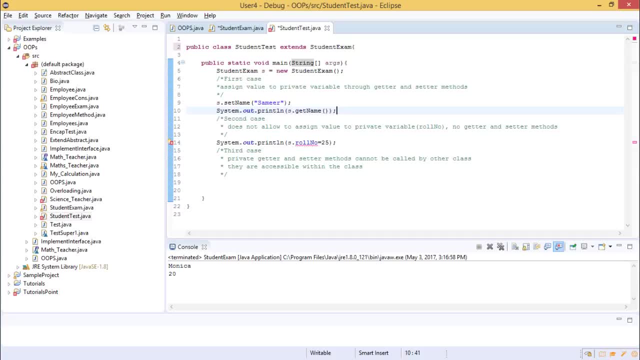 not allow you to assign value to private variables. So if you have not specified any access modifier, then you can call the private getter and setter methods, because there are no getter and setter methods for this particular private variable. Next is your third case, because, if you see, here we were. 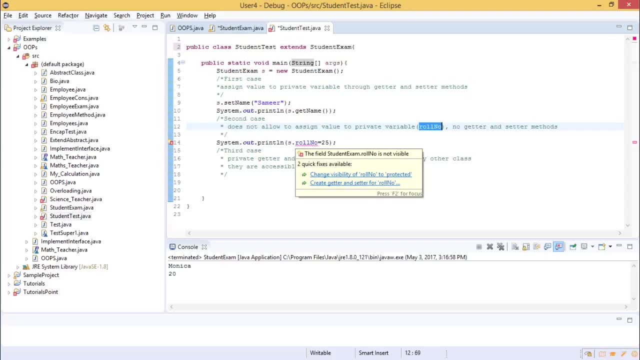 trying to change the value it says, change the visibility of roll number to protect it and create the getter and setter method for roll number. Why? because it is declared as private in our student exam class. The next one is private, greater and setter methods cannot be called by other class.